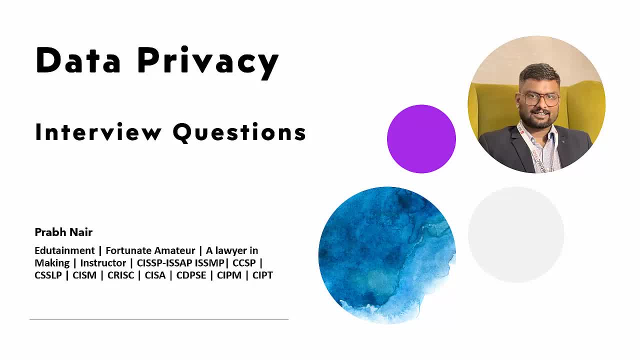 Hello team, welcome to my session on Coffee with Prabh, and today we're going to discuss some interview questions which is frequently asked in a data privacy jobs. My name is Prabh Nair and for more information you can check my LinkedIn profile. These questions I also ask when I basically onboard any consultant for the project. So might be this video useful for you And if you're new to the channel, do subscribe to my YouTube channel and click on the bell icon to make sure you should not miss my future videos on a similar topic. I also covered the interview. 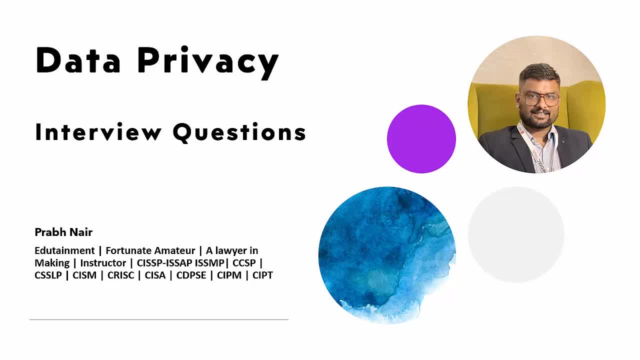 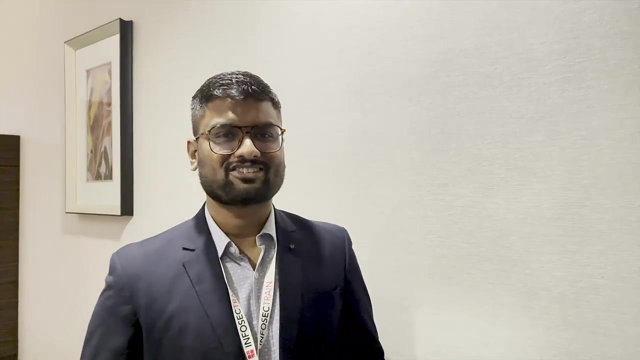 prep questions of the other job skill set. So might be that videos will be useful for you. My primary objective behind this YouTube channel is to just give a value to my clients, value to my stakeholders, value to my subscribers so that they gain information from this particular channel. So, without wasting your time, let's start with the first part. Hello everyone, my name is Prabh Nair and I'm working as a chief instructor at InfoSecTrain. 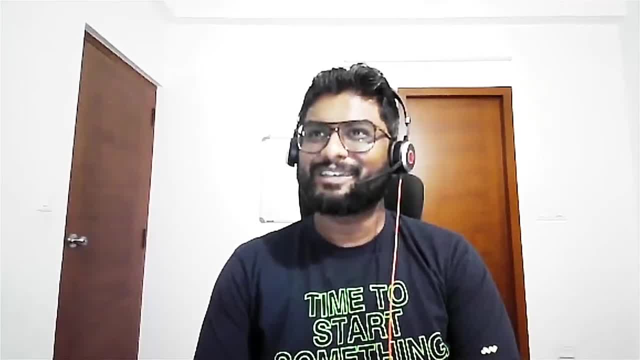 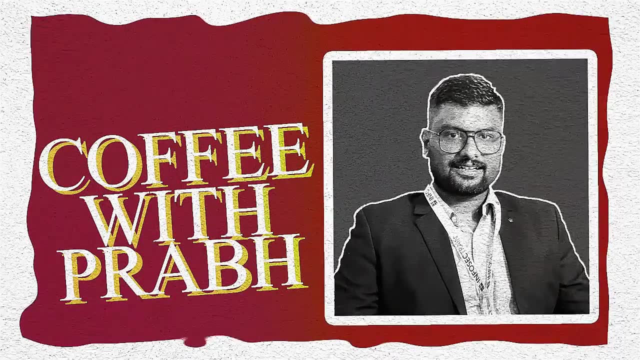 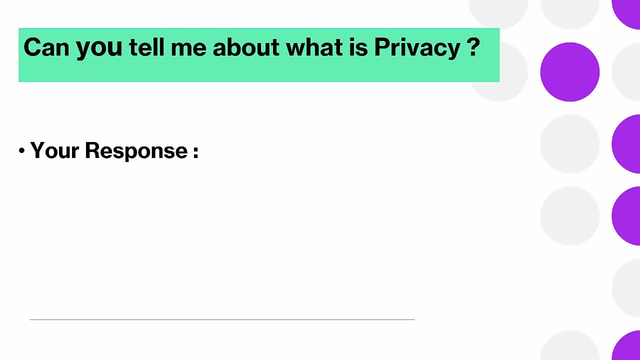 Okay, so we are starting with the first question. Can you tell me about what is privacy, or can you tell me more about what is privacy? See, normally, interviewer, when they ask this question from the candidate, they want to know the thought process of the candidate, Okay, what he basically or what she perceive about privacy, Because 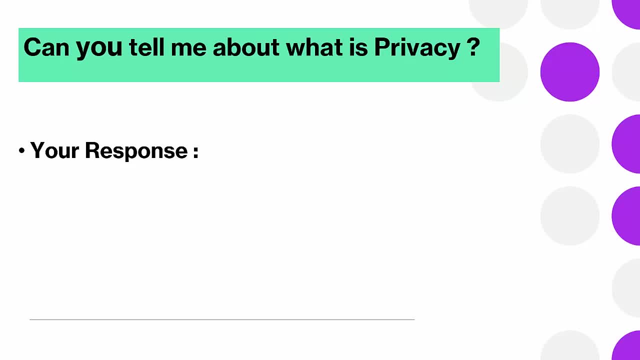 it is very important to know the psychology of the candidate, how he take or how she take the privacy as a subject. Okay, because privacy is a very complex thing. when it comes to their solutions and all that It's a very complex thing. So most of the interviewers normally ask this question just to understand what is the visibility the candidate has about the privacy. So if you are going to answer this question, or if I'm going to answer this question, this is the normal response I give to the question. So privacy is a state of 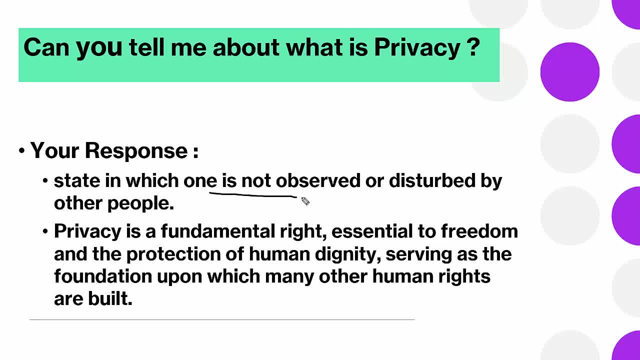 information in which one is not observed or disturbed by the other people. Example: like my medical records. So I have my medical records. Okay, I want that information only with me. So I have some medical informations. Okay, I went for some test and this is my information and is basically associate with me only. So I don't want this information should go outside to any third person, because that is a state of 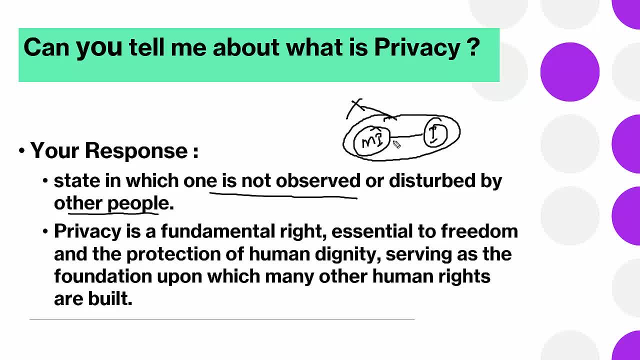 information for me And I might get disturbed if that information is available to third party because he might misuse that information for his personal benefit. That is why, in some countries, privacy is a fundamental right- Okay and essential to the freedom and protection of human dignity and serving as a foundation upon which many other human rights are basically built. So this is how you can able to present the statement. So if someone asks about what is privacy and why it is important, it's a state of information. 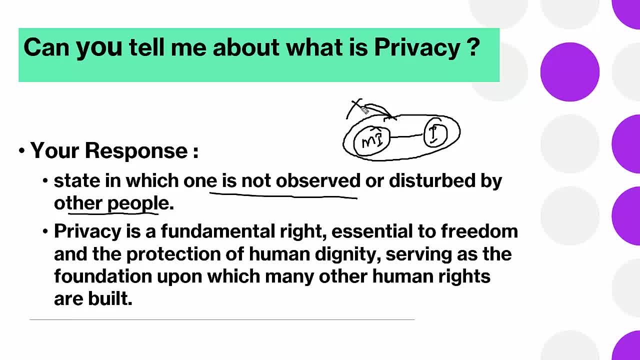 Which neither observed on disturbed, disturbed by the other people, and it is a fundamental rights in some countries, which is considered as a human dignity, And that is why in some countries we have a dedicated law which basically protect the privacy of our individual. One more important thing: sometime in the interview they also ask what is the difference between the privacy and secrecy. So privacy is a state of information which deal with the individual. 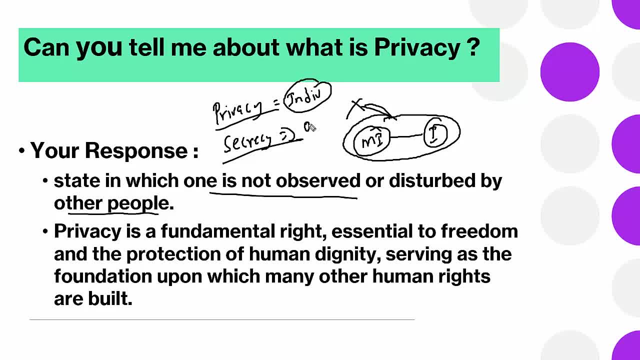 And secrecy is a state of information which deal with the organization. Example company has their internal business information, They have their internal trade secret. So that is called a secret information And the information which is mapped with the individual. that is basically called as a privacy. 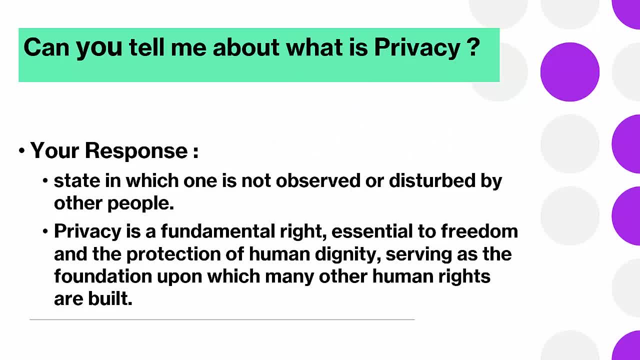 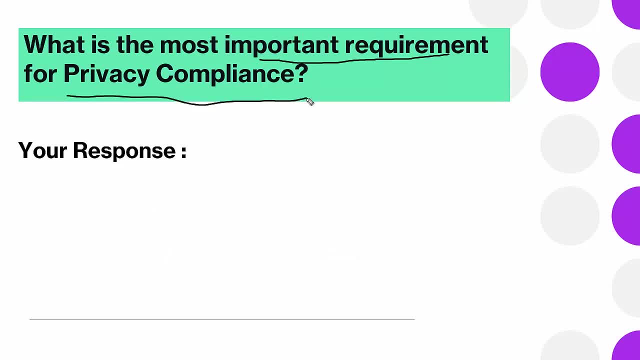 Okay, so let's move to the next interview question. Okay, next question is: what is the most important requirement for a privacy compliance? By asking this question, interviewer, want to know your experience in the data privacy area, Because you know they cannot hire any random consultant to manage a privacy because it is something related to their law, regulations, business requirement and all that. 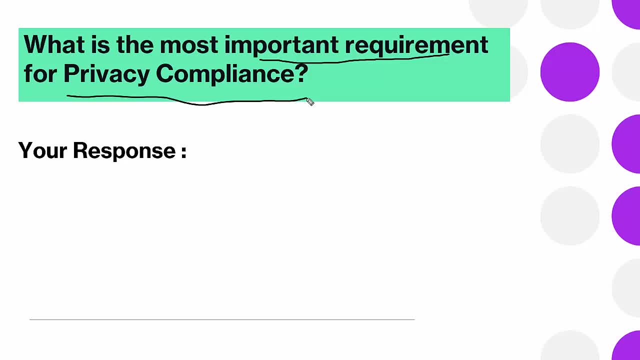 So they want to know your experience, they want to know your knowledge on that particular area. So this is how I basically craft this question. That's why we have raised this question: What is the most important requirement for privacy compliance? And, as a client, I will definitely ask this question from a candidate. 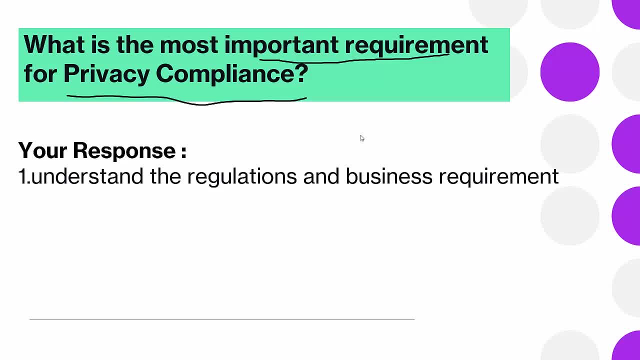 So answer is: first understand the regulation business requirement, Because if you want to start building any kind of a privacy system in the organization, we will definitely need to know: okay, what are the current requirement we have? what is the business requirement we have? let's take example: i joined one um european based company. okay, so this is the company we have. 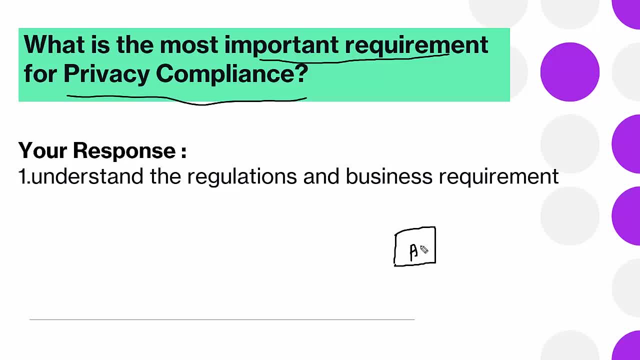 company a, so i joined this company, so i need to make sure that, okay, a company should be comply with the gdpr, or they have a customer in us, so i need to be comply with uh, hipaa, i need to be comply with glba, or, if i am basically serving any kind of a customer in canada, i need 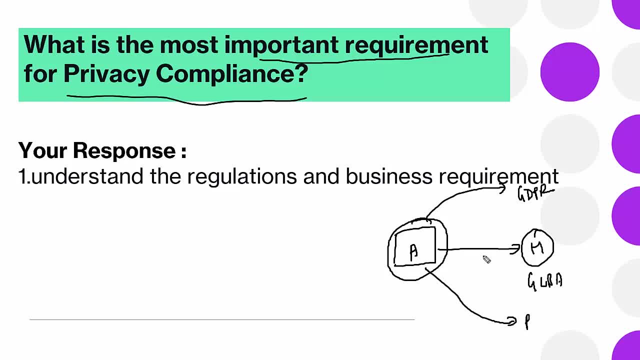 to be comply with the pipeda and all that. so, first thing, in order to comply- comply is basically mean act of abiding. so in order to comply with gdpr, comply with h epia and all that, i need to first understand the requirement. simple logic like: if i'm, if i'm going to someone's house, i need to. 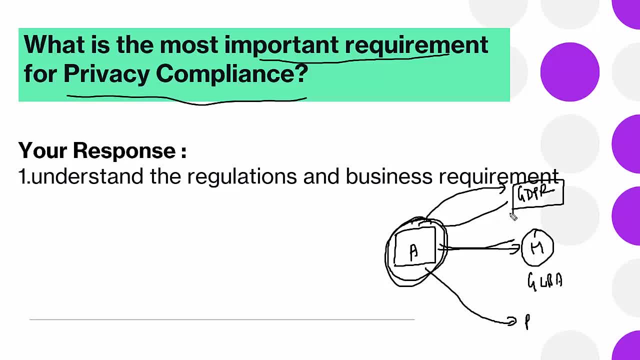 know the rules and the requirements, but before that, just understand their requirement. let me share an example in another way. let me take four steps if you want to know their requirements. regulation of the house- right, that is how i get the respect and that is how i get my safety. and 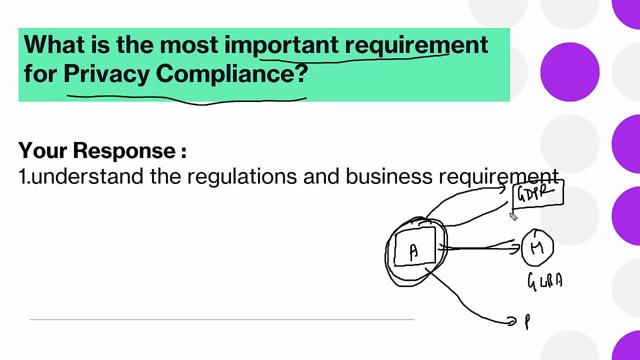 security same like as a company. if i'm basically operating in a particular region, i need to know their business requirement. i need to know the regulatory requirement of that particular region. okay. now if gdpr say that, okay, you need to process data in a pseudonymization. so i need to make sure. 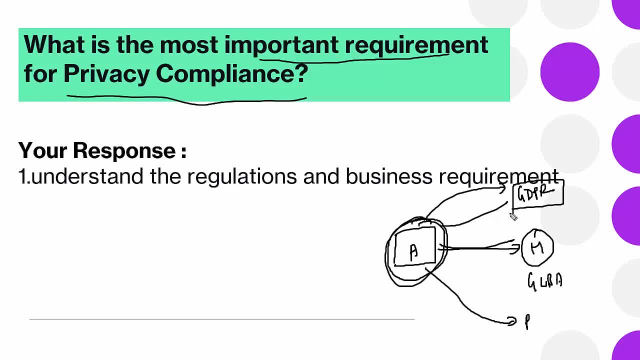 what are the data is processing in the eu, it should be done in a pseudonymization. if glb is saying that tomorrow you need to keep the data address in an encrypted order, i will keep the data in encrypted order. so before implementing the encryptions and all that, i need to know what. 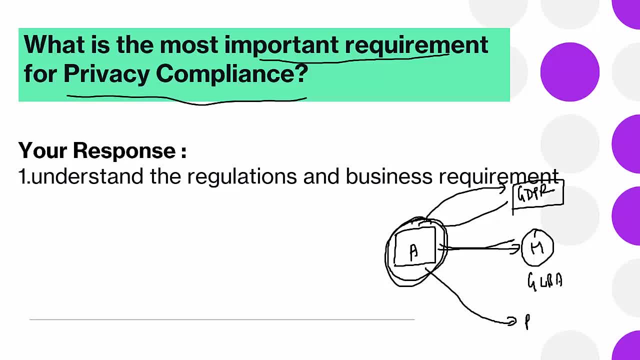 is the requirement. so that is why that is the first step. so when you're going to explain in this way, you build the confidence in the interview. yes, this guy has a knowledge. so second step: appoint the data protection officer. in some cases we need to have a data protection officer. he is just act like 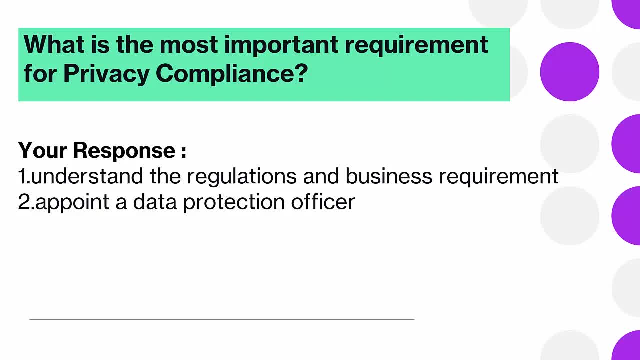 a data steward who understand the business requirement and map the business requirement with the legal requirements and he, he or she will be the person who will basically talk about what is the requirement we need to be comply with the privacy. okay, the third most important thing: we need to create a privacy. 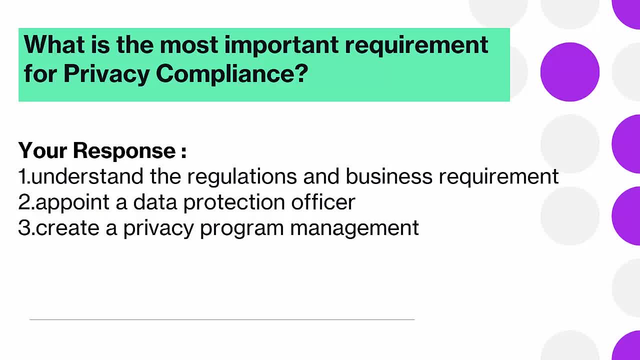 program management, because it include all the controls, procedures and everything by which we basically maintain the privacy protection. and then we basically create a privacy policy which basically capture the intent of the management, because if you want to enforce any kind of a privacy practices in the organization, it need to be driven through a privacy policy and then 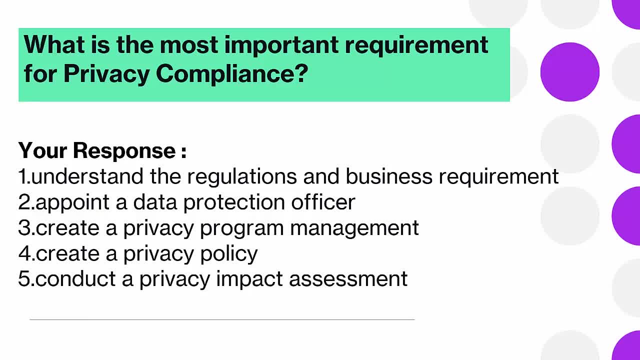 finally, we conduct the privacy impact assessment, which basically all about what is basically have and what we need to achieve. privacy impact assessment is just like a gap assessment to identify the level of privacy requirement we have in the process and what we correctly have. so this is how the process we follow, by which we can able to 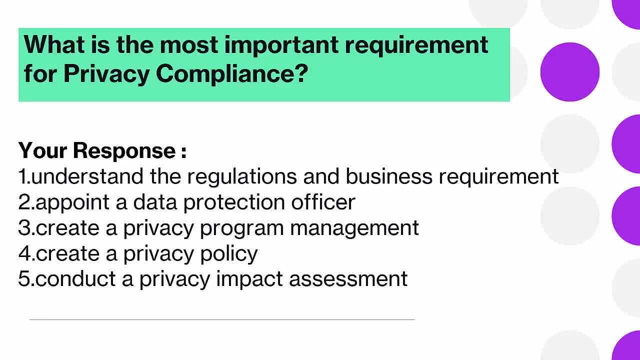 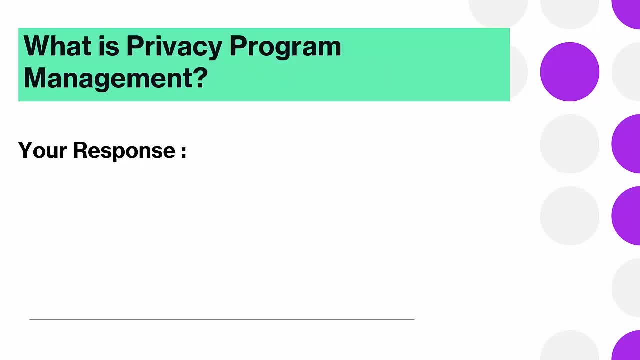 compliance with any privacy requirement. let's move to the next interview question. okay, next question is: what is privacy program management? frequent question. ask the exam. see the next interview is: what is privacy program management outlook- excellent quick question questions: see the next project question is: what is See the way we're creating a management system, ISMS- Information Security Management System. 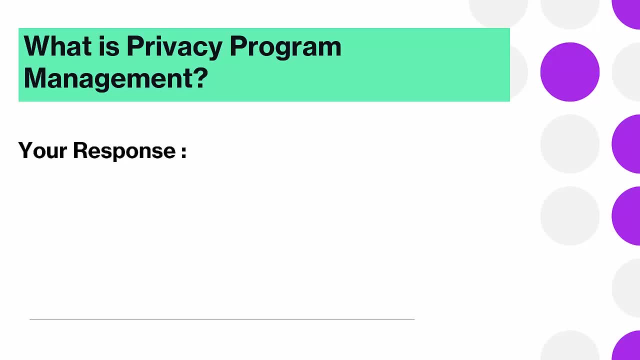 which basically talk about all the information security controls to protect the data and all that Same. like when we're building a privacy concept or privacy engineering in the organization, it has a set of controls, Okay, And for that that set of controls are organized in one particular. 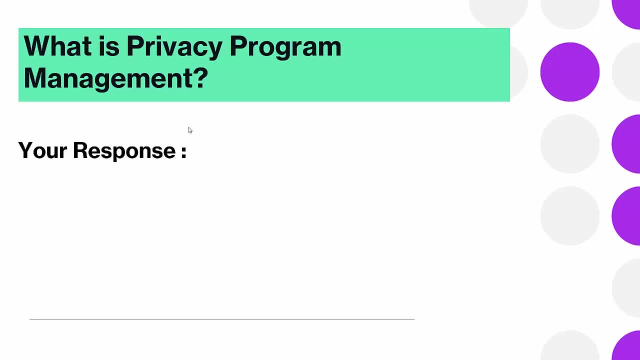 system And that system is called as a privacy program management. So privacy program management is a frequent question which is, you know, asked in the jobs and all that. So how you basically respond to that? So it is basically a comprehensive approach to privacy and data protection, that is. 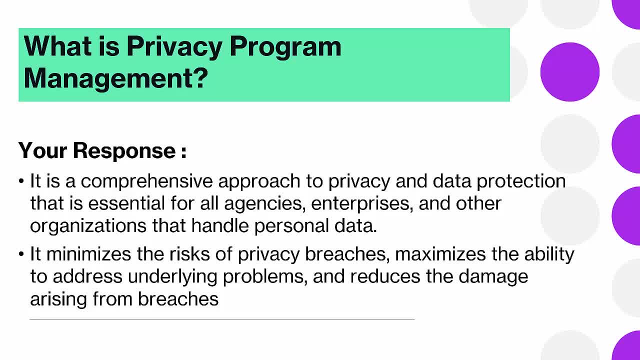 essential for all agencies, enterprise and other organization that handles personal data And it minimize the risk of privacy breaches, maximize the ability to address the underlying problems, reducing the damage arising from a breach. So, in a layman term, like: let's understand. 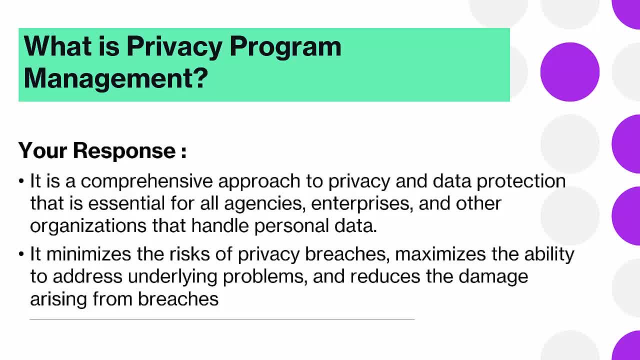 see privacy program is all about. you can say it's all about stablishing, stablishing, implementing and continually improving an organization private program to ensure we can basically compliance with the applicable data privacy regulations. So the way we have ISMS- Information Security Management System- 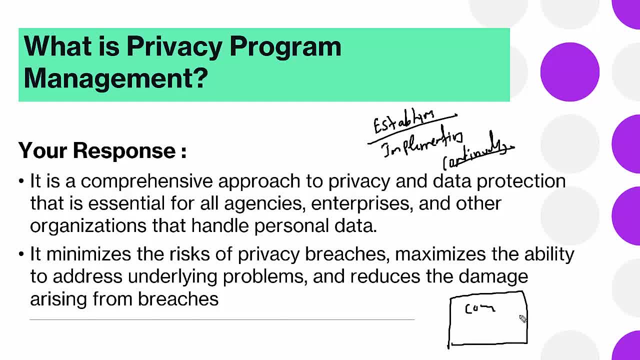 which basically includes all the controls and practices. Same, like I want to comply with privacy regulation, I want to comply with privacy requirement. So how to do that? So we basically build the system in which the policies are there, controls are there And that that concept is basically called as a privacy program management. Now, sometime, what happened? interviewer also asked what are the steps is basically required for effective privacy program management. So in that the first step is basically establish the privacy program. That is a first step. 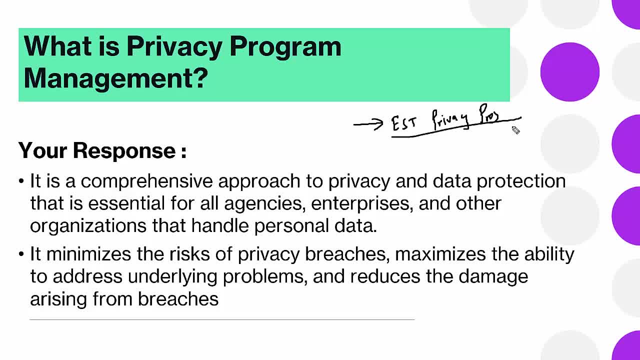 So we build the system, Establish the privacy program- Okay, Where we establish the program that define the organization approach to data privacy, set out the policy procedures, process for managing personal data. Then second step is basically we conduct the PIA. 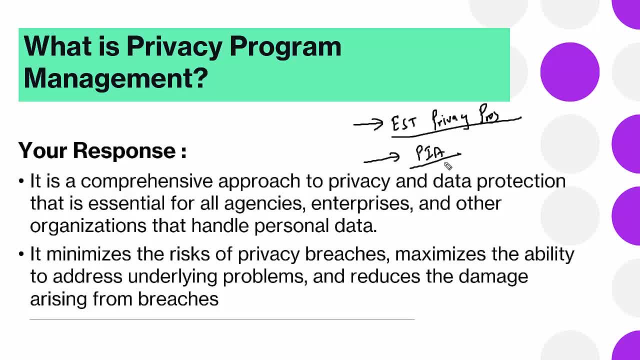 Privacy impact assessment or privacy risk assessment, where we perform the risk assessment to identify the potential privacy risk to the organization, personal data as a process, And then third step is basically called as a developed the privacy management plan. So this: we develop the privacy management plan that outline the organization strategy. 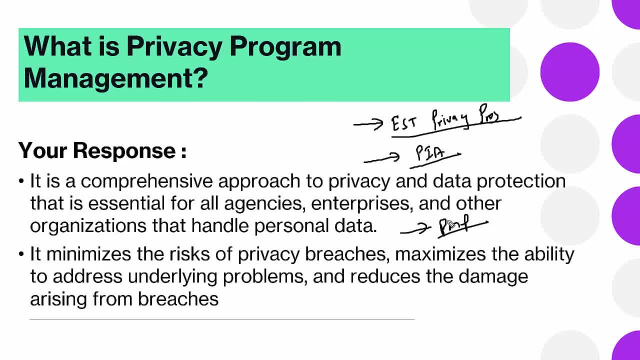 for mitigating privacy risk and compliance with the applicable data or any regulatory requirement. and this plan should include all the privacy control process and procedure. So that is what privacy management program is all about: it include the controls that we need to apply, include the processes and, most important, include the procedure. and then 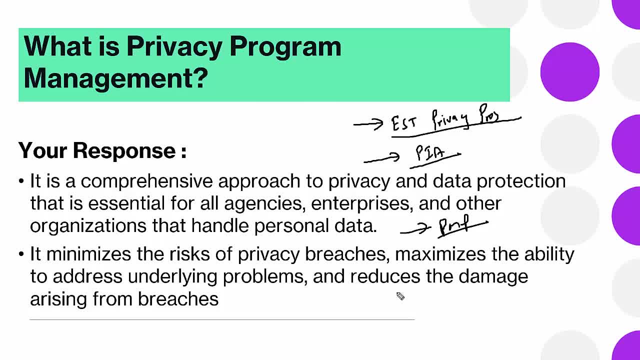 once we create that, the next thing what we have to do is we need to implement the privacy controls. Implement privacy controls. so implement the privacy control is all about identify in the privacy management plan, and this include implementing technical controls such as encryption, access control and all that. and once you basically implement the control, the next thing we have 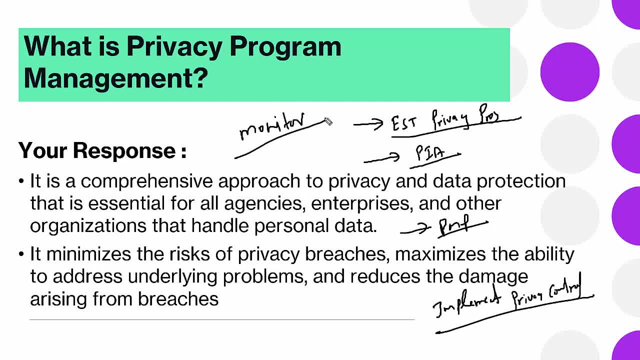 to do the monitor. Monitor is basically all about monitoring the effectiveness of the plan, including your privacy control process, to ensure you know ongoing compliance with the applicable data privacy regulation. Then we need to have an incident response plan where we develop and implement the incident response plan to respond to the privacy incidents and we need to train people on the privacy. 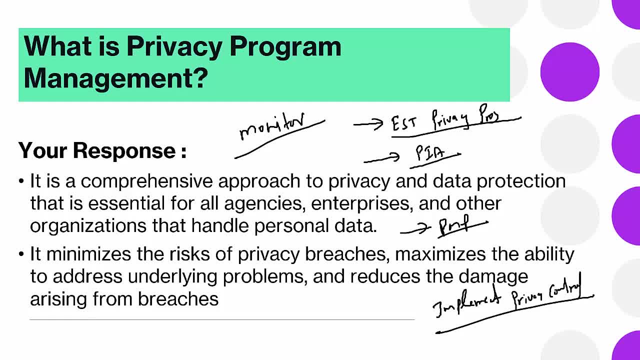 activity. So somebody is established the privacy program, then conduct the PIA, then develop the privacy management system, then implement the privacy control, then monitor and then we have a train and review. So this is how you basically build the privacy management system in the organization. 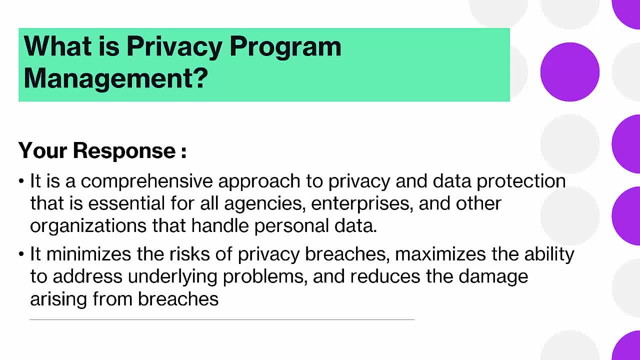 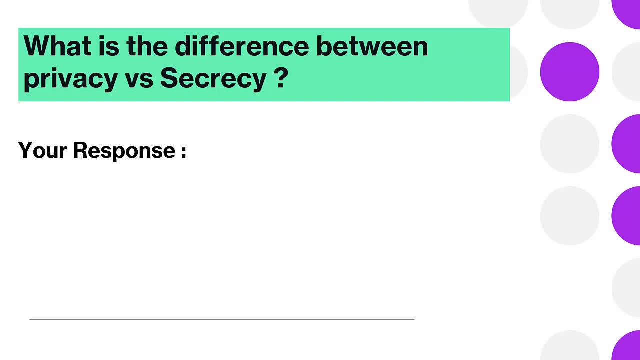 So it include the set of activities. it include the set of controls, process and procedure which talk about How to maintain the data privacy in the organization. Okay, let's move to the next interview question. as I said sometime, interview trying to confuse you with the very basic questions, because you should be good in basics and this is what 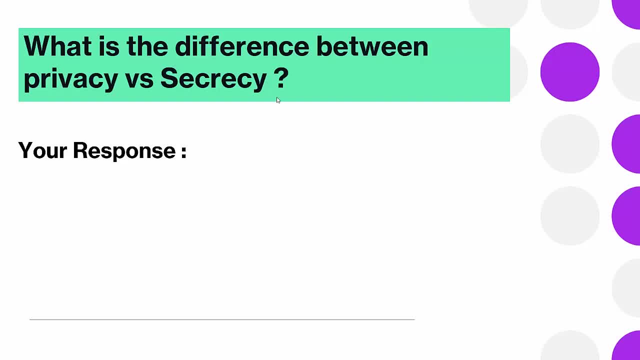 the basic question is: what is the difference between the privacy versus secrecy? So privacy is a state of information that deal with the individual, like your PII, your health records, whatsapp chats and all that Okay, which is something little individual. And secrecy is a state of information which deal with the enterprise example, like companies. 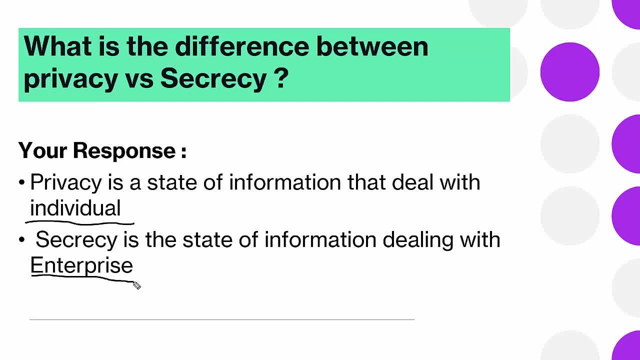 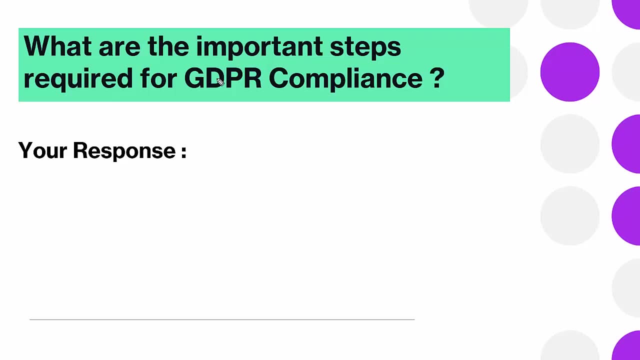 business process and all that. So that is the thin line difference we have between the privacy and secrecy. So let's move to the next interview question. Okay, next question is: what are the important steps required for a GDPR compliance? Now here I basically divided the response into two part: one is very high level and one 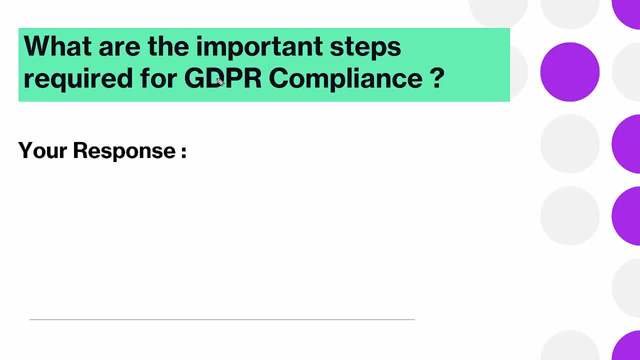 is basically detail level. Now The interviewer basically asked this question a different way. example: we already have a compliance with other regulations, but you know we don't want to repeat the same step. so do you know any high critical steps that we can consider, by which we can even directly? 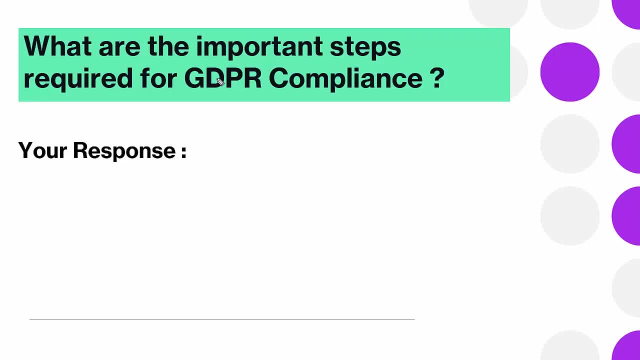 comply with GDPR, Or you know what are the important critical steps are required to be comply with GDPR on a high level. So this is basically where the interviewer test your experience. they want to know your experience in the GDPR area. so I have divided the response in two part. one is very high. 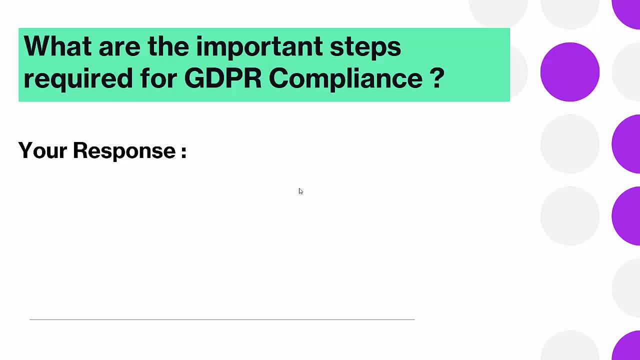 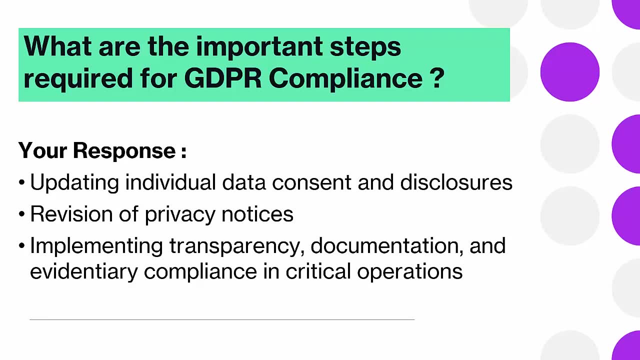 level And the second part is very detailed level. So high level is updating the individual data consent and disclosures. normally current process we have, which is compliance with PIPDA and all that, but according to GDPR, we need to update the consents. Current policies, privacy notices are compliant with PIPDA, so we will update all the necessary. 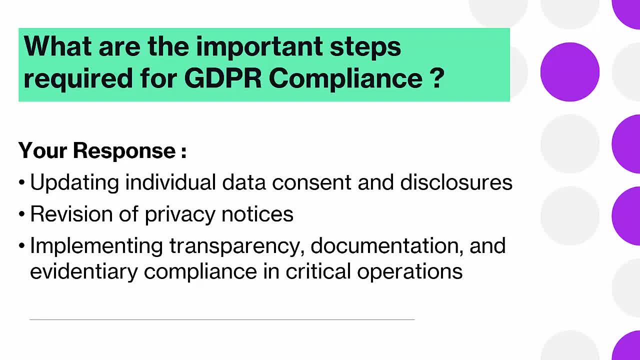 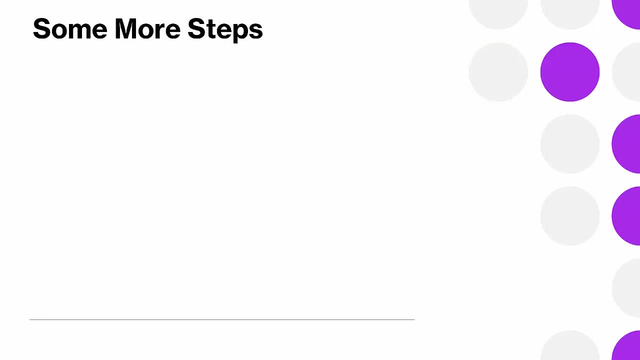 requirement of GDPR. and third is: implement the transparency documentations. okay, whatever the critical documents are required to be comply with GDPR. I'm going to update instead of going from a scratch. So that is basically very high level steps. Okay, If you want to know in detail, then I have also a step for that example. like the first, 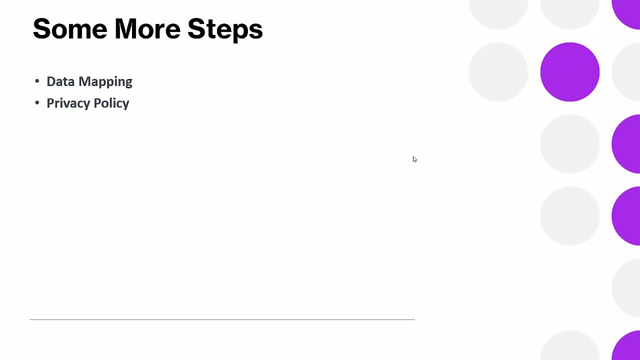 step is data mapping: okay, where we identify, map all the personal data okay, which we collect, the process, store, including the category of data location. you know the legal basis for processing it. that is the first step. Then we basically create a privacy policy. we need to develop and implement the privacy. 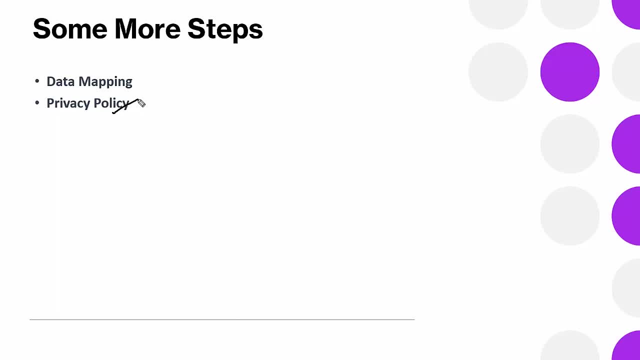 policy, because privacy policy is a foundation of a privacy governance. okay, always remember any kind of a system program We want to introduce in the organization. the first we need to create a policy for that. so policy is a law and order of the company. okay, so develop and implement the policy that. 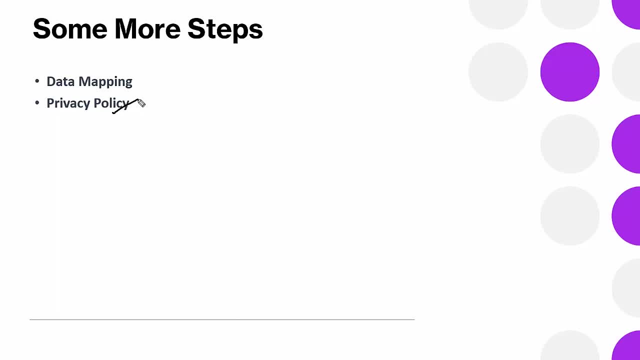 inform individual about how the data is collected, how it going to be processed and how it going to be shared. Then, third important thing, we need a consent management, so where we need to establish the processes to obtain and manage the consent from the individual for collecting, processing. 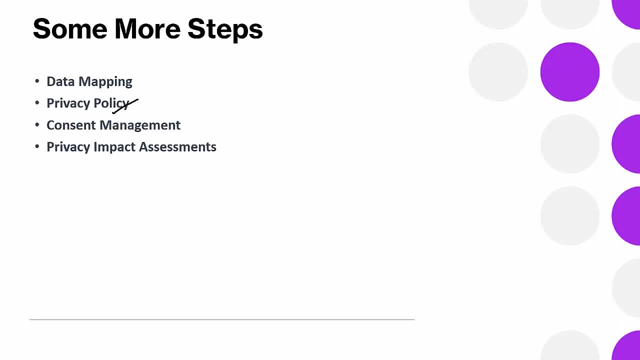 storing the personal data, how you going to process the data, so that is required and then once, Then we need to identify the gaps, and that is basically where the PIA come into the picture. PIA is one of the most important part of the privacy management system because it conduct. 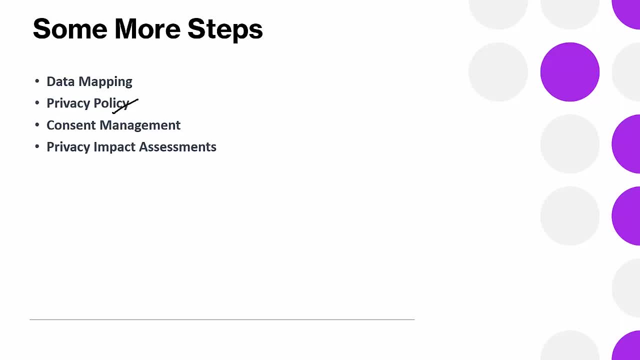 the assessment like. they identify the risk, they mitigate the privacy risk associated with the new project or changes in the existing process. let's take example: we are companies already compliance with other regulations and now this company is planning to onboard a new project, So they will try to understand what are the requirement of this business. okay, what is? 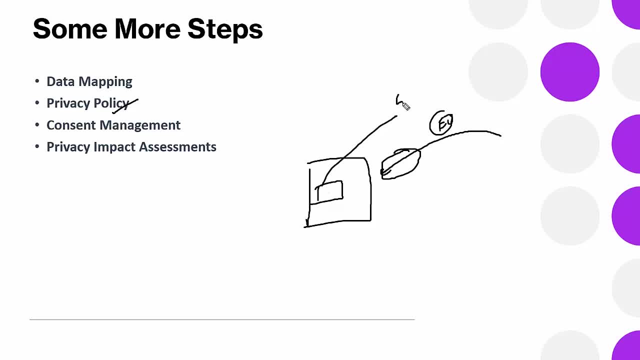 current control we have and how we can basically comply the GDPR. so let's take example: we have a website which is basically collecting a set of information from the Canada, and our website is comply with Canada. now we are planning to launch this website in the Europe, so I need 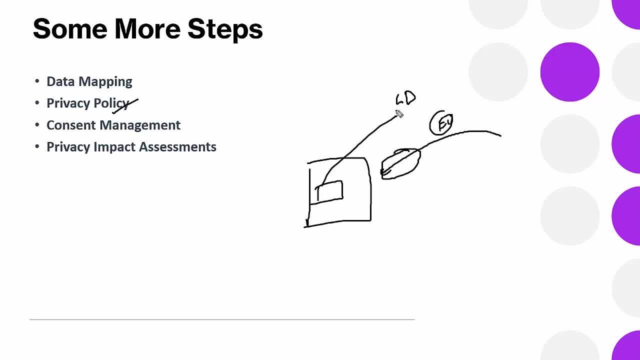 to see what is the set of requirement we need in the website. okay, so that we can compliance with the GDPR. Okay, so we identify the risk. oh, there is no consent mentioned. there is no privacy notice mentioned. this is how we did the PIA. okay, so user want STTP. so if I use STTP, there is. 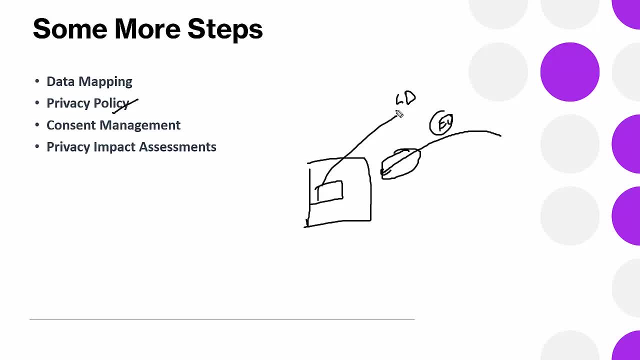 a information disclosure. so this is against the principle of GDPR. so this is how I am doing a PIA. So if you give such kind of an examples, it build more confidence. So PIA is the most important thing. so once we done with the PIA, the next step is basically: 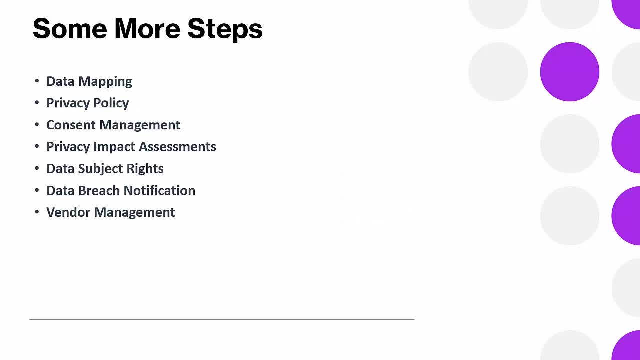 data subject rights. so data subject right is all about you know, implement the process to manage the system. data subject rights, including the how he access the data, how he rectify, how he erase the data, restrict the processing, data, portability- all this thing need to be defined. then we have a data breach notification in GDPR, the mandated report. 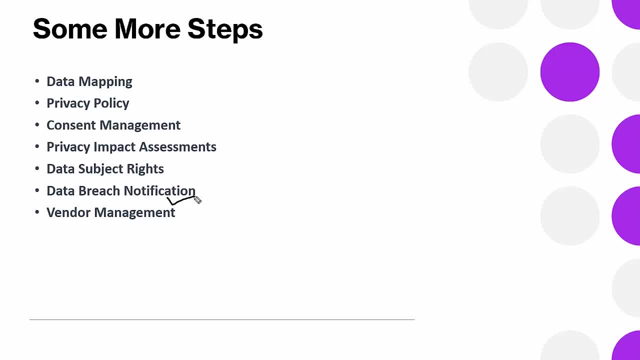 breaching is 72 hours. in 72 hour you need to report the data breach. so data is notification. we need to establish the process here to inform the individuals and all that sometime what happened. we onboard the vendors also and we need to make sure the vendors also compliance with your privacy when there should be. 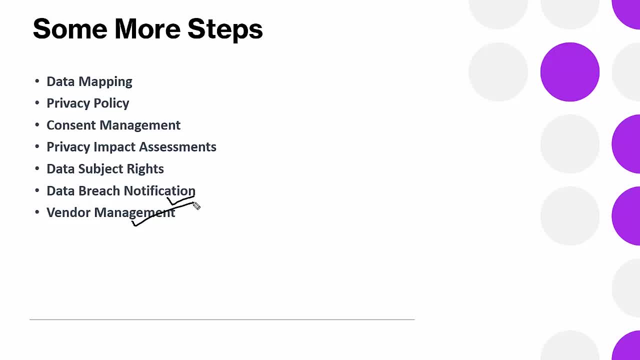 compliance with GDPR because, by end of the day, you are the one who accountable for the regulatory. so we need to implement the process to ensure the third party vendors compliance with the GDPR requirement when processing the personal data on behalf of the organization. then we have our training. 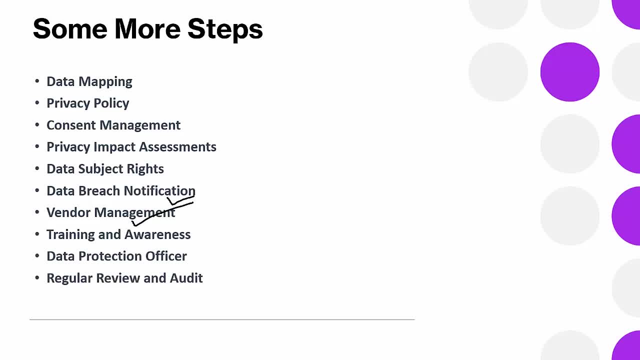 and awareness where we provide the regular trainings to the employees to ensure they are under GDPR requirement. and then we have a minimum appointment of data protection officers- okay to oversee the GDPR compliance and they should be served as a point of contact with supervisory authority and regularly audit and review. 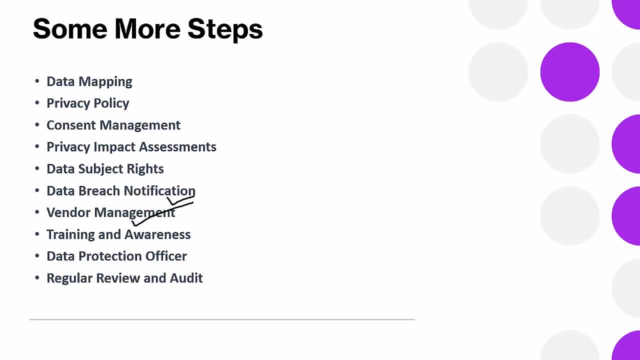 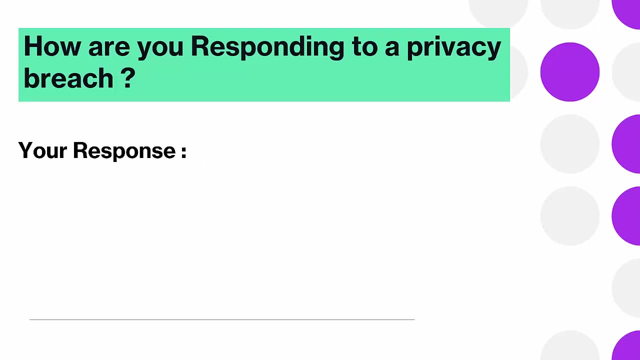 just to make sure we are compliance with all the GDPR requirement. so these are the detailed steps we have by which you can able to comply with the GDPR. okay, let's move to the next interview question. okay, how are you responding to the privacy breach? privacy breach it means if sub tomorrow, any breach happen, how you going? 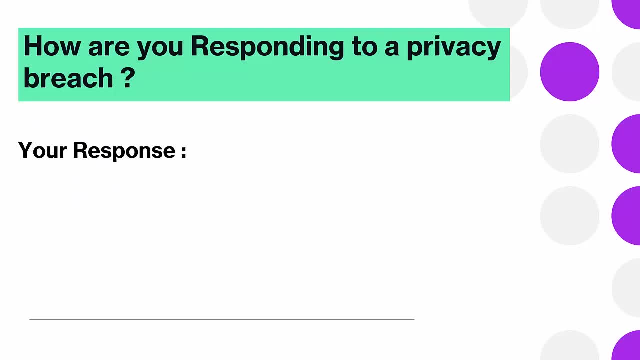 to respond to the breach, because here the interview- want to know your psychology of how you handle the crisis. okay, how good you are in handling the crisis because failed to comply with privacy, or if there is a privacy breach you need to phase a regulatory compliance penalties and all that. so here want interview, want to know how you basically 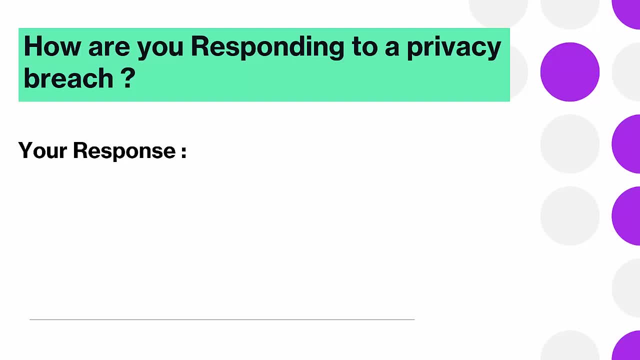 handle such kind of a situation. so how are you responding to the privacy beasts of? first is: contain the bridge. contain the baby's example if system is in fact it with the virus. isolate a system immediately from the network. that is my first priority, instead of doing start. 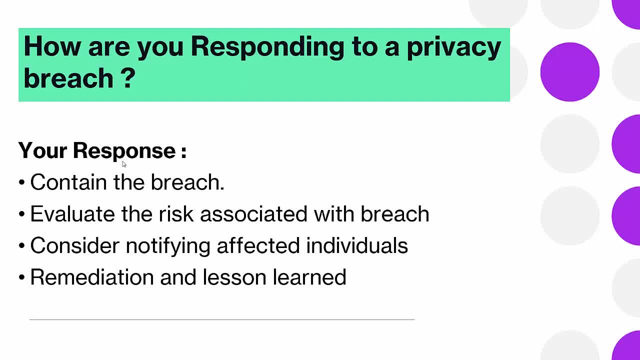 doing a troubleshooting there itself. so example like: we have a server here and Okay, and these servers are basically connected with the other servers. So the hacker example like hacker hack into the server and able to access the data. But I don't want further damage. 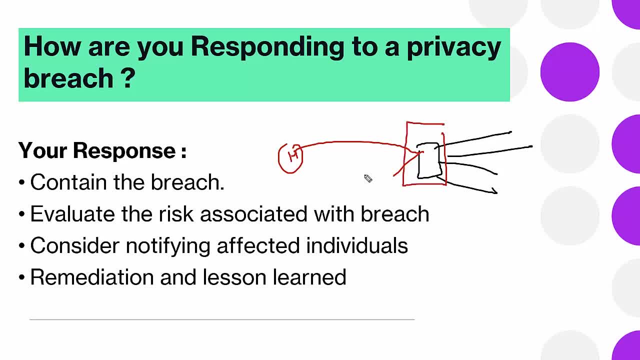 So isolate a system from the network. that is the first thing, And for that I will first notify the incident response team and they will basically isolate a system immediately from the network And then we do the further investigation: how they hack the system. 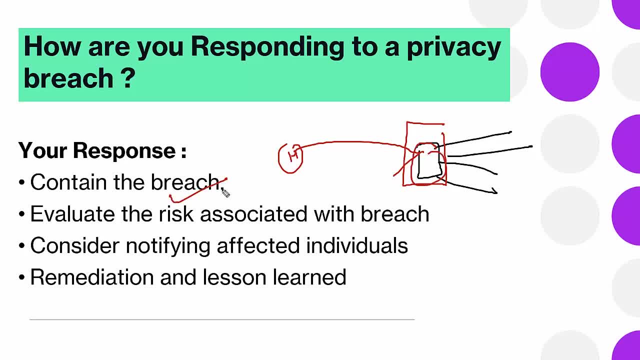 So that is called as a contain the breach. It means limit the breach. Second is: we will evaluate the risk associated with this breach. Okay, what is the level of affected things we have? So, example: 20% of our data got compromised. 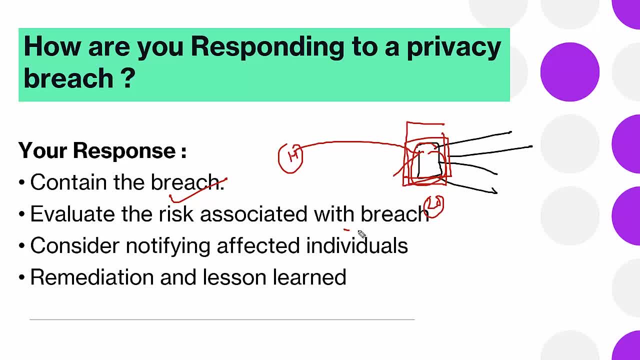 So at least we save 80% of our data here. So we evaluate the risk associated with the breach. Okay then, according to GDPR, I need to report the breach. So I will see the. what is the notification requirement we have? I will basically get: 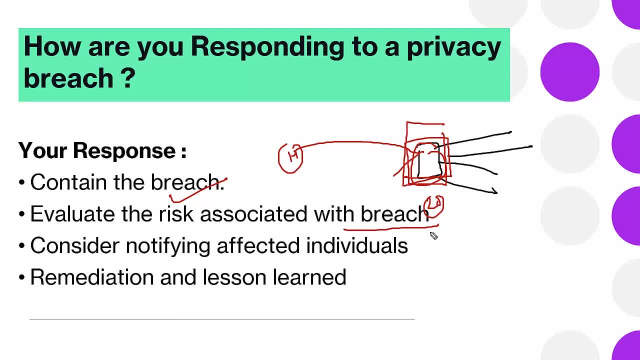 it done, the plan PR team will be involved. how to craft a message And then we basically proceed with the remediation lesson learned. Remediation lesson learned: make sure this incident should not be repeated again in the future. So that is how we basically do the problem management, root cause analysis and all that. 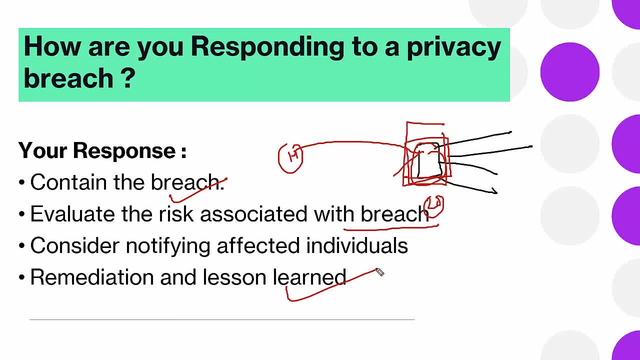 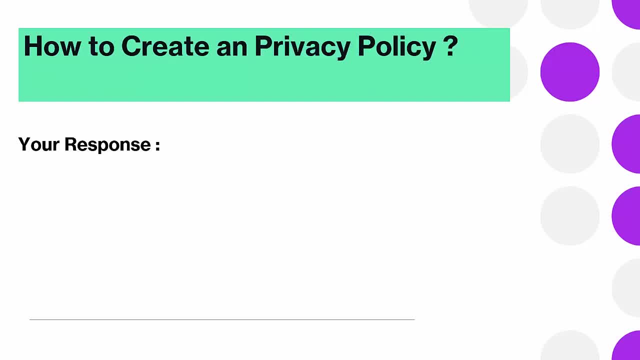 So that is how I'm going to respond to the breach. Okay, next interview question. Very good question: How to create a privacy policy Here the interviewer- how to create a privacy policy Here the interviewer- want to know whether you are good in writing and all that, or you. 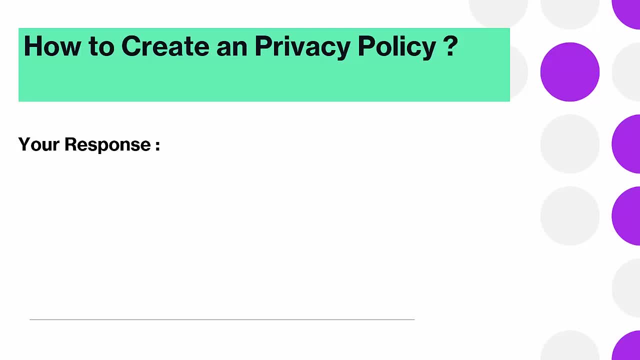 have a good understanding of governance and all that. So the first step, Whenever you're creating a policy, is to understand the business and legal requirement. One thing you need to understand: privacy is a foundation of any governance. okay, Management intentions are covered in the policies. 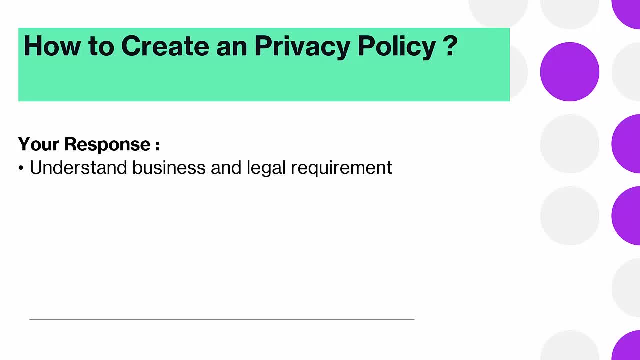 Okay. so, example: every system must be protected with the password. So this is the statement, come from the management, So that is a policy. So whenever you want to build a privacy governance, privacy management, privacy policy is a mandatory step because it is created by the protection officer and approved by the senior management. 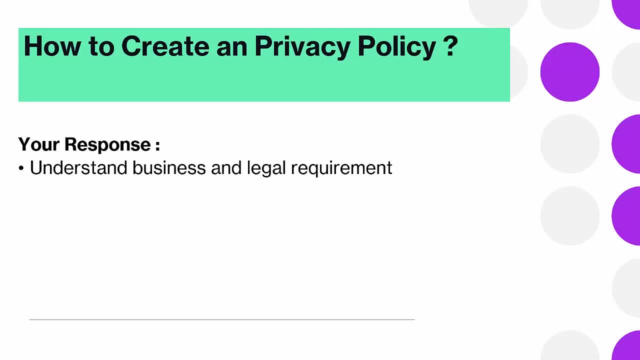 And whenever you're creating a policy, Make sure the policy capture all the business and legal requirement. That is the most important and must as a category. Then second is define the scope and statement. okay, like this policy is basically applicable for which country or policy applicable for which branch or policy applicable for which? 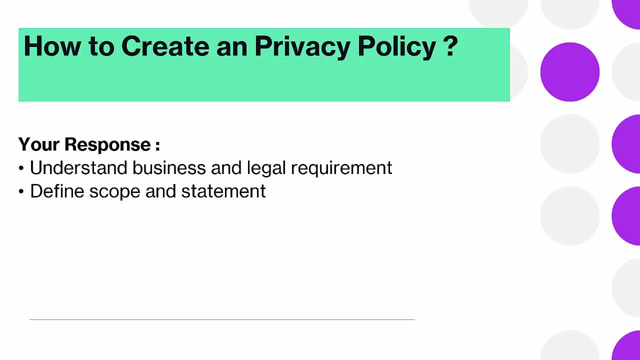 business process. So, example, like we are the multinational company where we have a project from Canada, we have a project from us. So, according to us, we need to create a privacy policy for us process. we need to create a privacy policy for the GDPR. 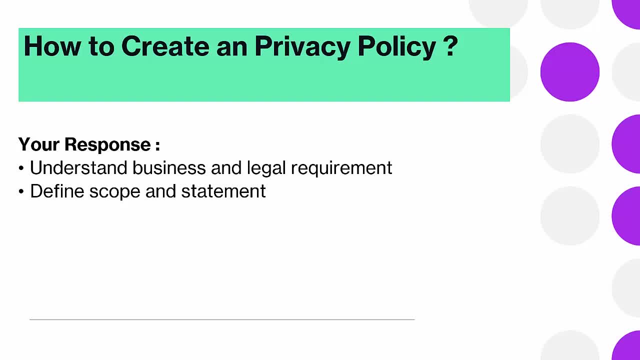 We need to create a privacy policy for the GDPR, We need to create a privacy policy for PIBDA. So we need to define here: is this policy applicable for which particular area? So that is why the scoping is very important. Otherwise it is difficult for the people to follow. 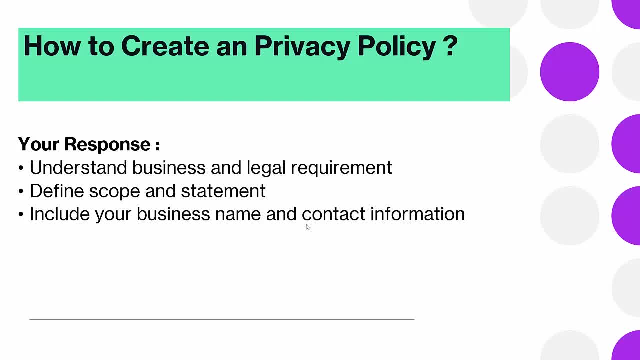 It is very important to include your business names and contact information. So if someone- if tomorrow is someone- is confused with the policies and all that, there should be a point of contact that the person can reach out. mention about what type of information you're going to collect in the policy. it is very important define what type of information. 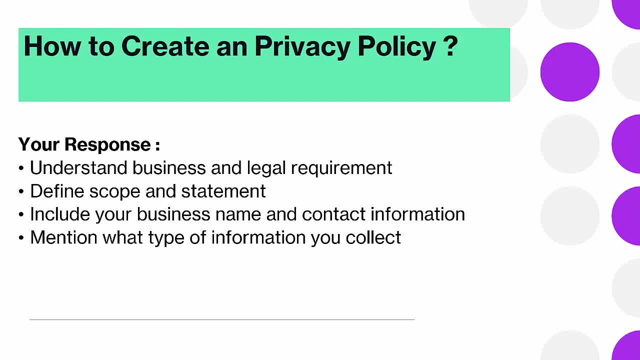 you collect. Okay, There are many different way we collect the user information. example like contact form, cookies, survey course registrations, you know, email newsletters. So this is something we need to define, need to address how you're going to collect and why. 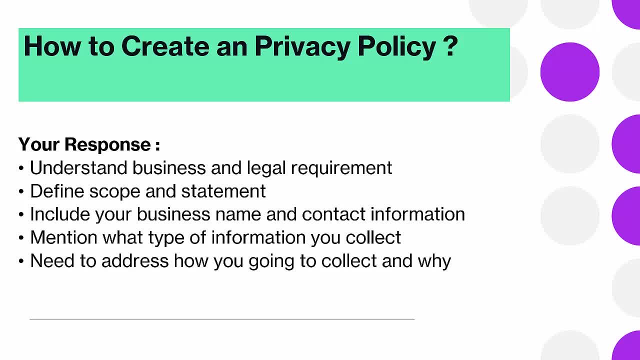 So it's very important Define the procedures okay, because it gives the clarity what, why we need that. And last, need to define if user data is shared with a third party. if yes, mentioned that and, last but not the least, for how long you're going to collect the data, because by this 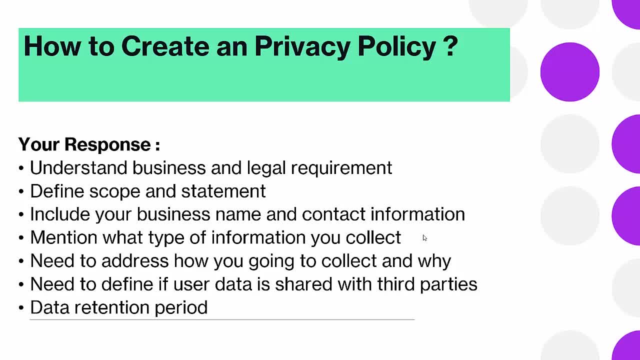 is how you can able to limit your liability, Because you have collected data and you're keeping the data in the database and tomorrow it got hacked, then you are answerable for that. So define the retention period for how long you're keeping the data. 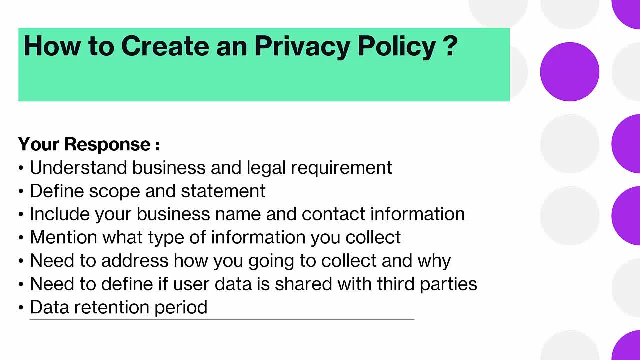 Okay, so by this way, you can able to limit your liabilities. okay, because we have a one simple fundamental is: the best way to protect yourself from any kind of a compliance issue is limit in the collection of data. Okay, let's move to the next interview question. 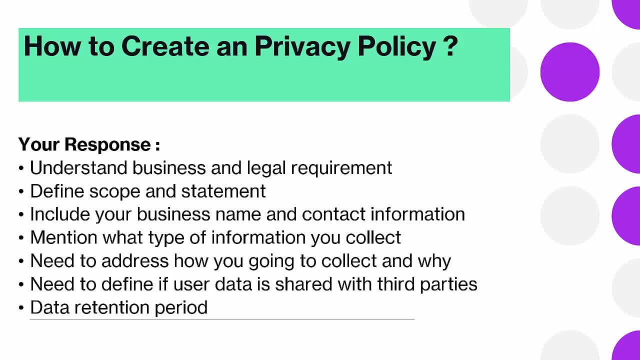 Before moving that, there's one more important thing: Policy need to be reviewed annually. Okay, Policy need to be reviewed annually or, in the case of major change in the business and policy, when it reviewed annually, it need to be reviewed with the version update. 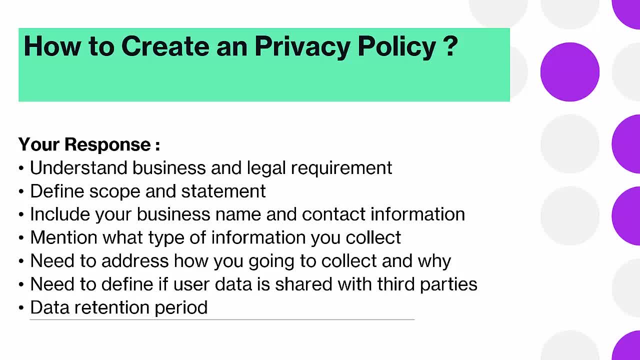 So in the last page there is a called as a version update, like policy was revised on this particular data And this is the version information. okay, We also need to add the policy exception process example. sometimes things are goes against the policies or sometimes we have to drive some activity against the policy. 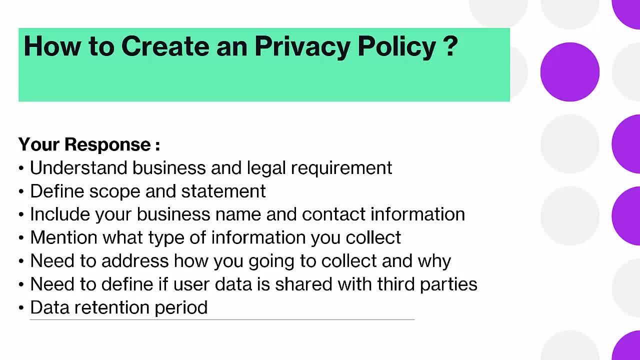 So we need an exception approvals and that also need to be tracked down And later on annually we'll see how many times this kind of an exception has been generated And if it is basically generated multiple times, try to amend that in a policies. okay. 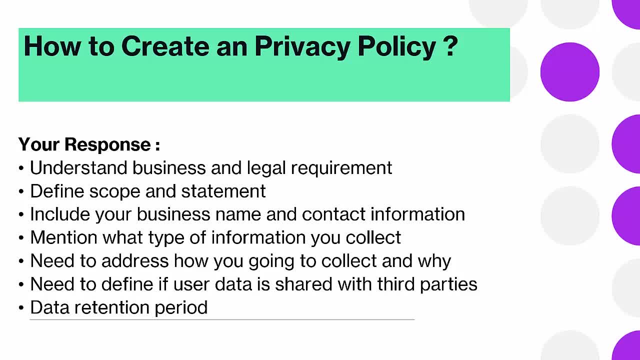 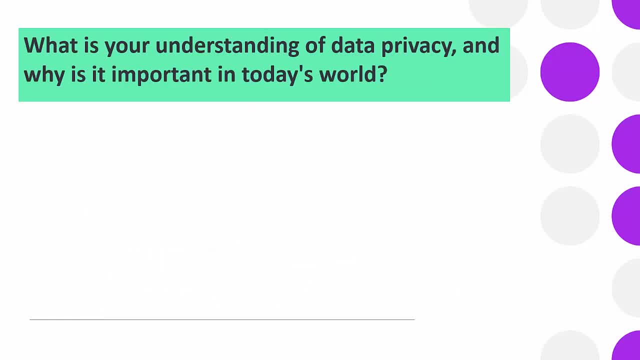 Now next thing is next interview question is: what is your understanding of data privacy And why is it important in today's world? Sometime, the interviewer want to know your psychology behind the data privacy. okay, Because it is very important until and unless you don't have that state of mind to understand. 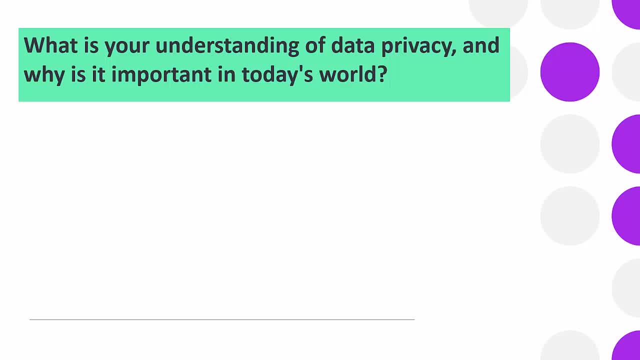 the privacy, you cannot be able to implement the control. That is why I'm going to talk about data privacy. Okay, So the first question was also on the data privacy introduction. So how you basically respond to that- See when you're talking about your response- is very simple. 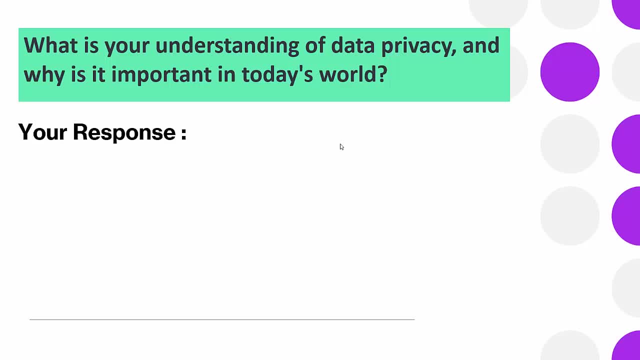 So data privacy, first of all. you give the definition, like data privacy refer to the protection of personal information from unauthorized access, use, disclosure, And then you can add some narratives here. like in today world, where the personal information is frequently collected, shared process, data privacy is critical to ensure that you know. 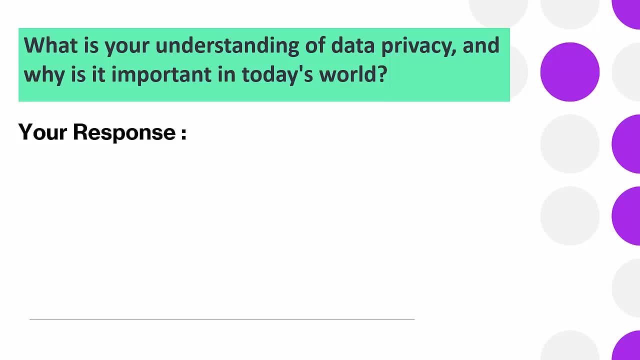 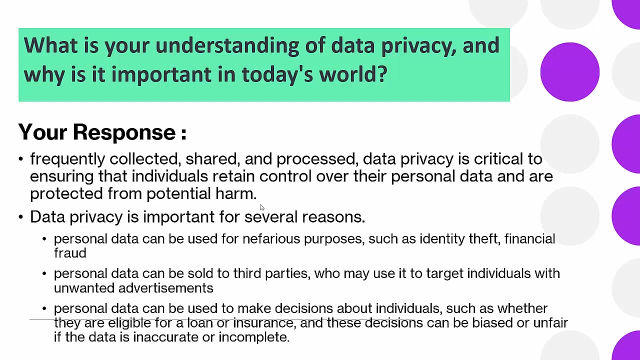 individual retain control over their personal data and are protected from the potential harm. This is how you can basically start the statement. Then you can give your observation like why data privacy is important in today world is first, personal data can be used for nefarious purpose, right? 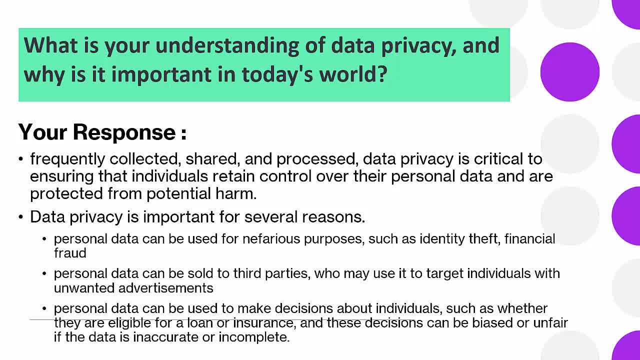 Such as identity theft, financial fraud or staking. That's why it's very important to have a data privacy. Second, is personal data can be sold to third party, who may use it for target individual. That is what we need to protect. 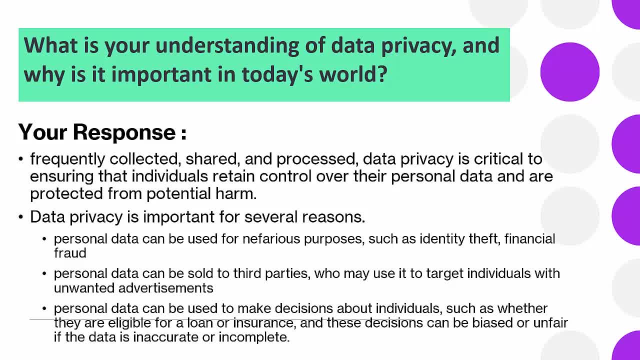 And third, personal data can be used to make the decision about individuals, such as whether they are eligible for the loans, Insurance and all that Okay. So overall data privacy is essential to protect the individual right, maintaining trust in the institutions and business that collect the personal information and ensure the personal 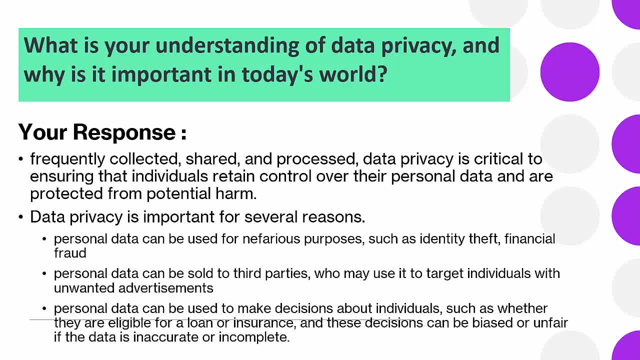 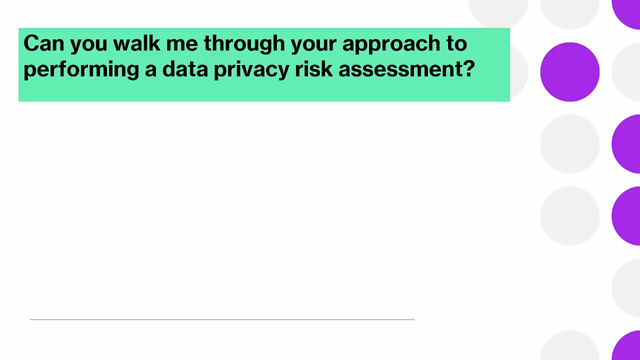 data is used ethically and reasonably. So when you give this kind of a narrative answer, I'm sure it builds the confidence in the job. So, sometime what happened? the interviewer also ask your experience on the data privacy risk assessment. okay, Because sometime what happened? whatever mentioned in the book is different from what is happening. 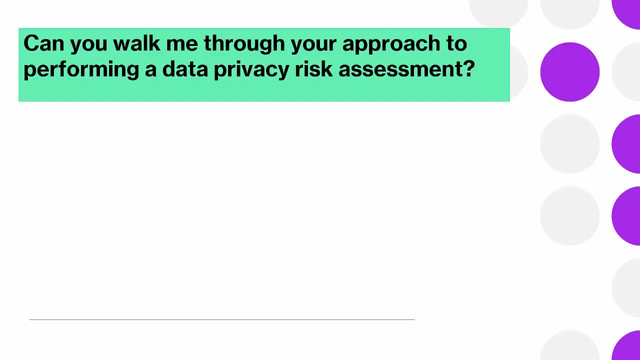 in the industry. Okay, So they will ask you sometime like: can you walk me through your approach to performing a data privacy risk assessment? So how you start, Certainly here is a general approach to perform the data privacy risk assessment. The first is identify the scope and purpose of assessment. 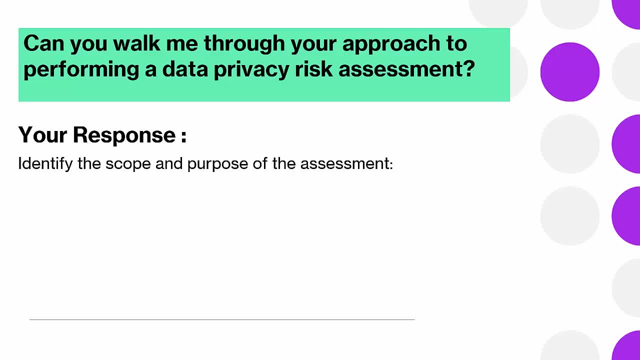 The first step in data privacy risk assessment is to clearly define the scope, the purpose of assessment, And this includes identifying the system, applications, data that will include in the assessment, as well as objective of the assessment. Second, is we need to identify the personal data? 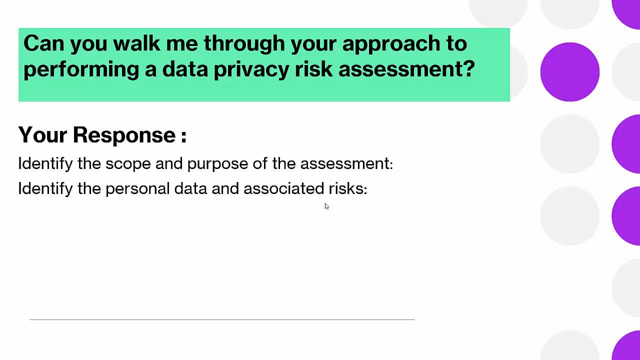 Definitely what data we have we need to assess, okay, which include analyzing a sensitivity of a data, potential impact of a data breach, unauthorized disclosure. Third, evaluating the existing control. That's another important thing. We will be reviewing the existing policy procedure, technical controls. 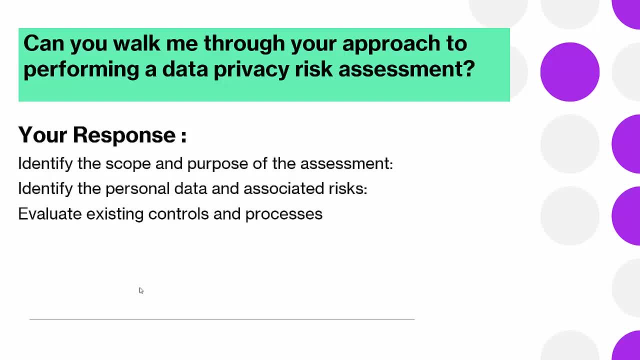 Do they are adequate? Then the next thing is identify the gaps, what we have and what we need to achieve. Okay, So, based on assessment results, we identify gap in the current controls, Like example, I did the assessment of the website. 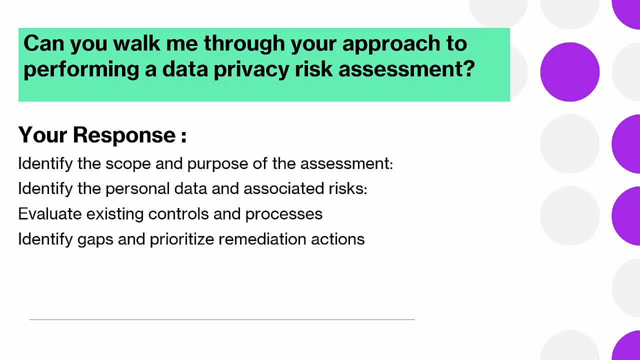 I discovered they are using SSL. What is required is TLS. Okay, There's no multi-factor authentication required. multi-factor authentication. So that is how I identify gaps, because a good privacy consultant doesn't mean, okay, start from scratch. When we already have some control, we need to just enhance those control. 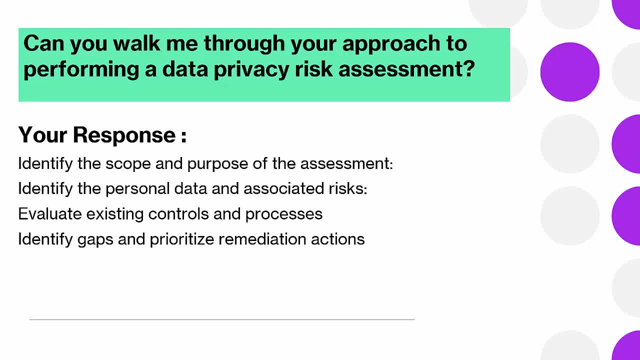 And that is how you can able to save the budget also. So identify gaps and prioritize the remediations- Is it clear? And then, based on that, develop the action plan. So when I say develop an action plan, it outlined the remediation actions: timeline, responsibilities. 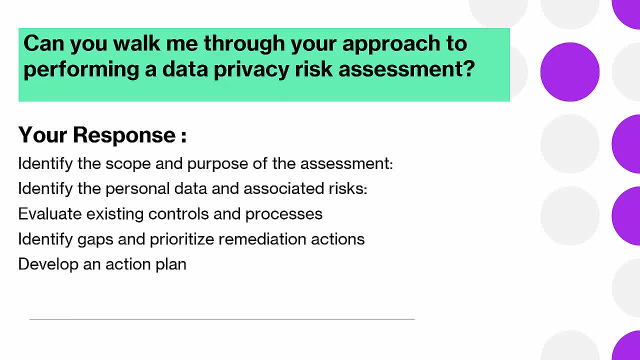 That is the most important thing, Okay. And then, finally, we have a monitor and review where we basically monitor the current control in place. So this approach can be tailored to meet the specific need and requirement of organization that applicable to the data privacy regulation.